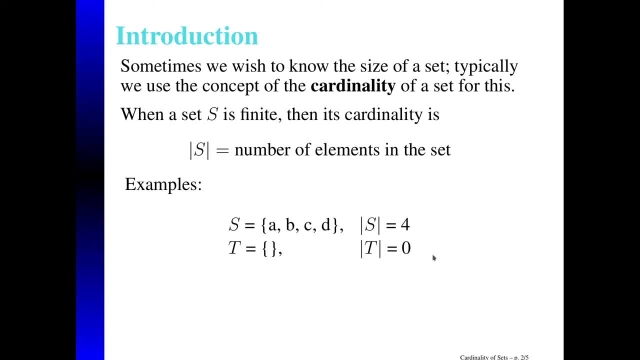 I don't see anything and therefore the cardinality of the empty set is zero. When we're discussing finite sets, the size of the set matches up with what your intuition probably is. That is, I'm looking to say: well, how many things? 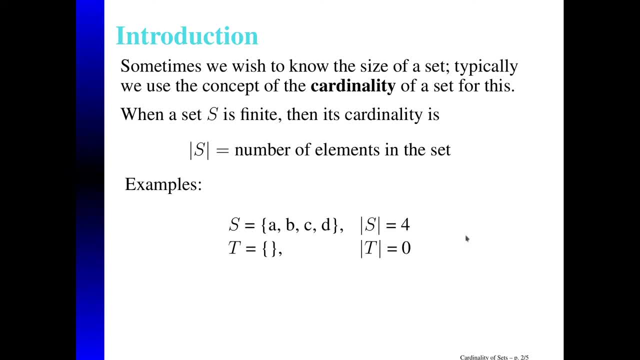 are in the set: One, two, three, four. Okay, that's what the cardinality is. It turns out, though, that when we're talking about the cardinality of an infinite set, it's not necessarily what we might expect it to be, And, in fact, we can have two sets that both have an infinite number of elements. 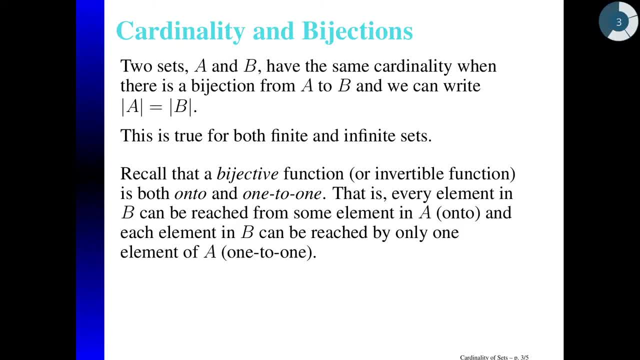 whose cardinality is not the same. Before we look at that, though, let's talk about another way to think about cardinality, And that is that two sets, A and B, have the same cardinality when there's a bijection from A to B. 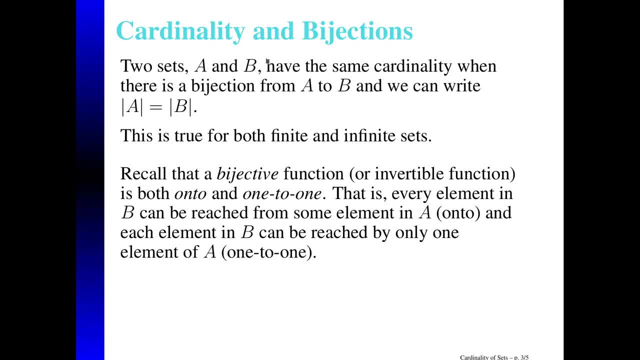 and we'd write it like this: The cardinality of A is equal to the cardinality of B. This is true when we're talking about finite sets or infinite sets. all right, If you haven't seen my video talking about sets in terms of or functions, excuse me, in terms of set theory. 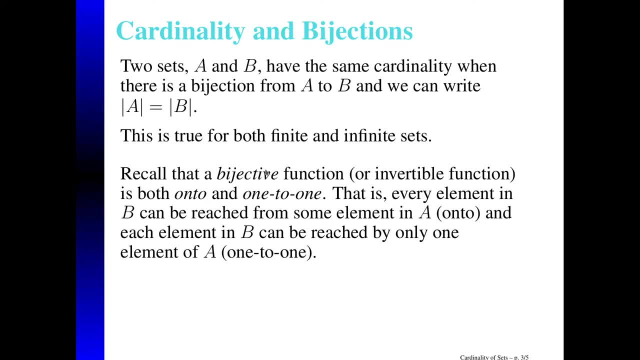 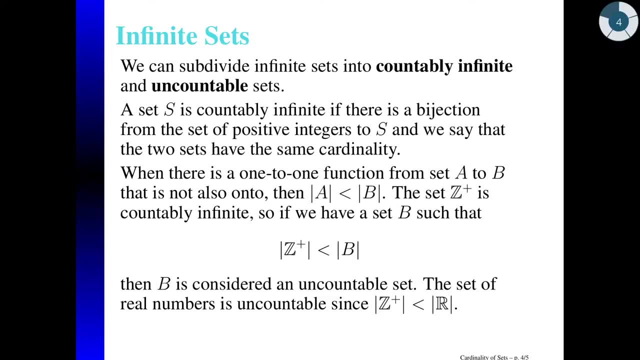 in which I discuss the definitions of bijective function, surjective functions and injective functions. you may wish to go back and look at that, But this sort of sums up what we're talking about here. When we are talking about infinite sets, though, we can divide those into two subsets. 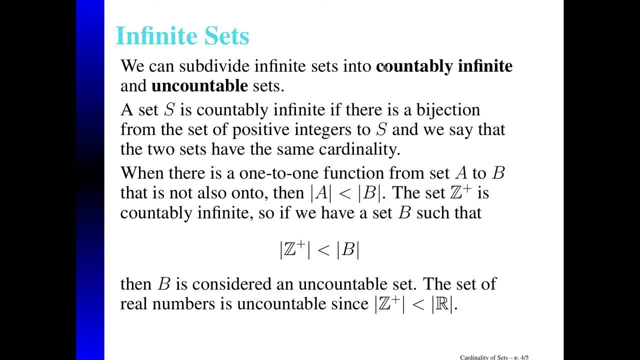 And those two subsets are those infinite sets that we call countably infinite and those that we say are uncountable. So a set S is countably infinite if there's a bijection from the set of positive integers to S case. we would say they both have the same cardinality. Recall that a bijection means that. 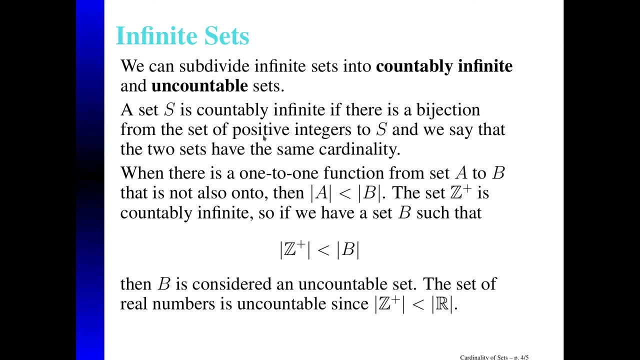 the function is both one-to-one and onto, So if we have a one-to-one function from set A to set B that is not also onto, then we don't have a bijective function. In that case, though, we would say the cardinality of A is less than the cardinality of B. Notice, here I'm not putting an. 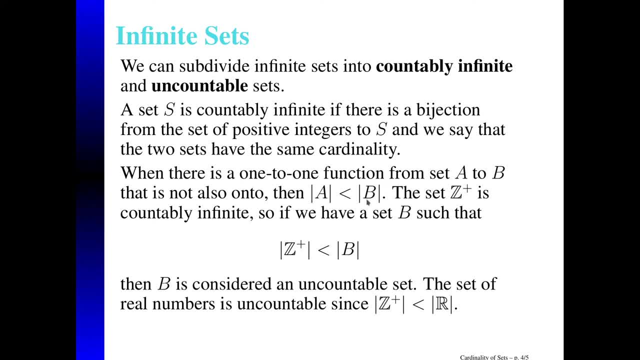 actual number to it, because if we're saying A has an infinite number of elements and B has an infinite number of elements, I can't really put an actual number to this. I just know that this cardinality is smaller than this cardinality. Now the set of positive integers happens to be: 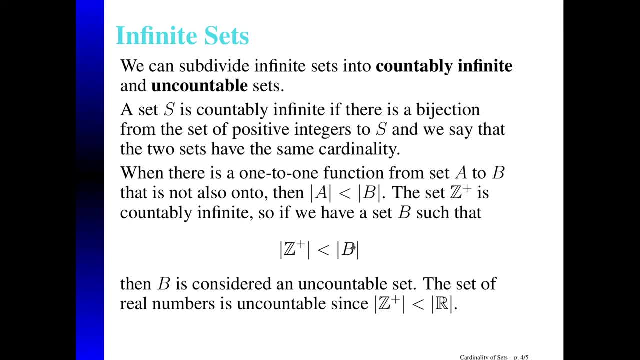 countably infinite. So if I were to have a set B whose cardinality is larger than the cardinality of the set of positive integers, then we would say that set B is an uncountable set, And that happens to be the case for the set of real numbers. Its cardinality is larger than the 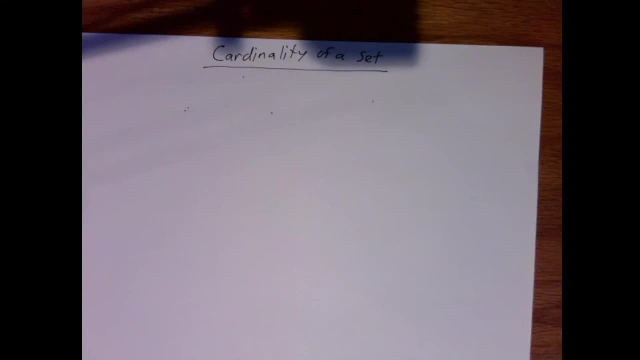 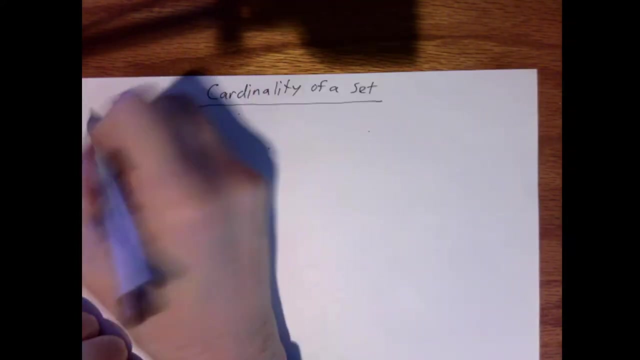 cardinality of the set of real numbers. So if I were to have a set B whose cardinality is larger of the positive integers, Let's revisit, though, the idea of the bijection from the set of positive integers to some other set. So this is true, The set of 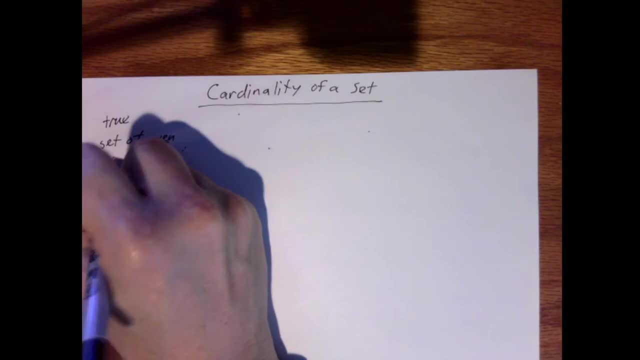 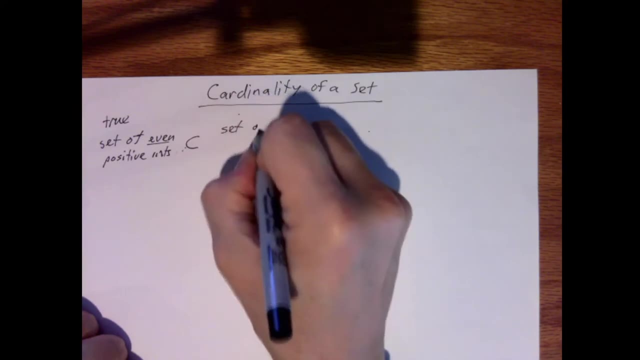 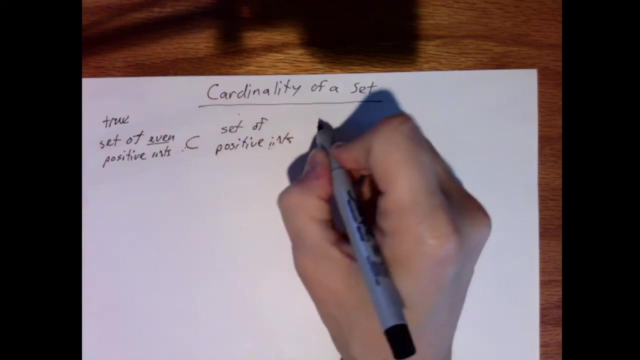 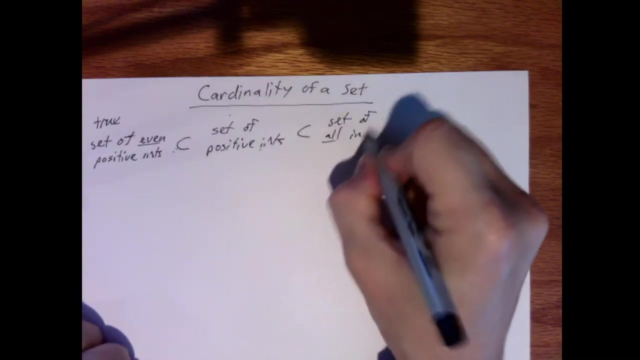 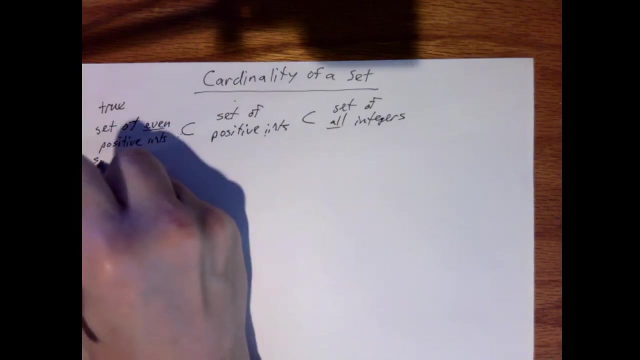 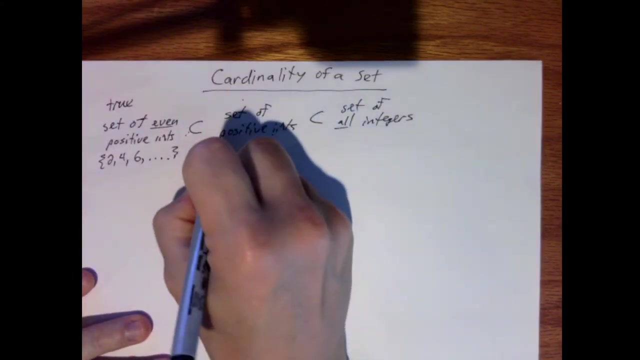 even positive integers is a subset of the set of positive integers, which itself is a subset of the set of all integers, which we normally say is just the set of integers. So what we're talking about here, the set of even positive integers, that's two, four, six, dot, dot, dot, The set of positive integers. 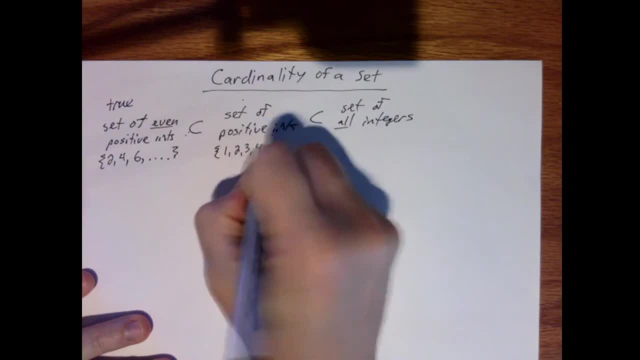 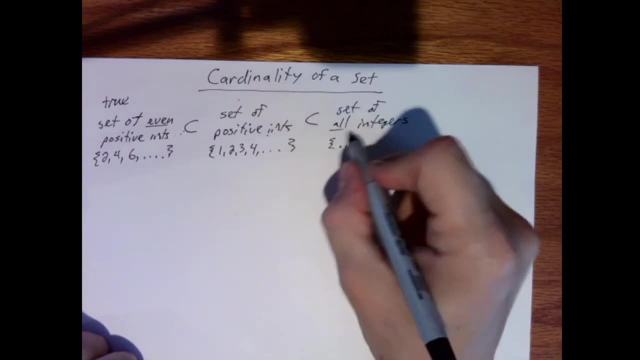 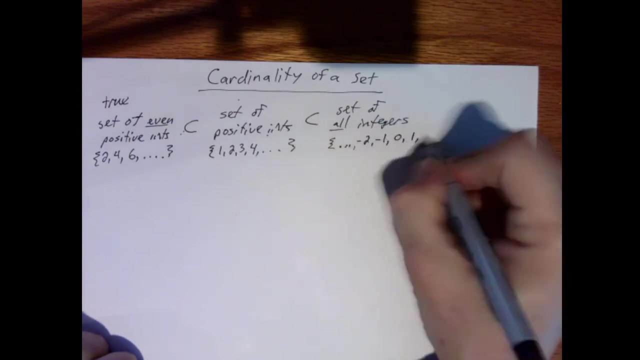 that's one, two, three, four, dot, dot, dot, And the set of all integers would be dot dot dot, because we have negative numbers going in the negative infinity direction: minus two, minus one, zero, one, two, dot, dot, dot. This is true, This is. 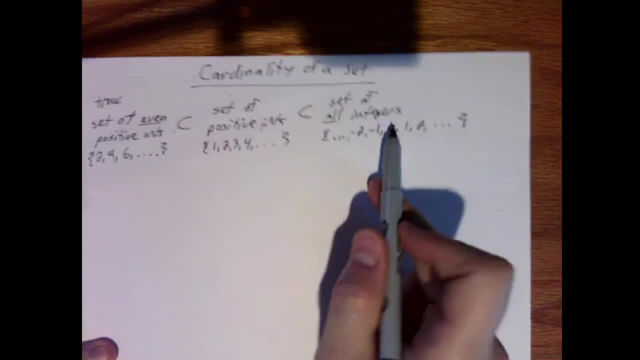 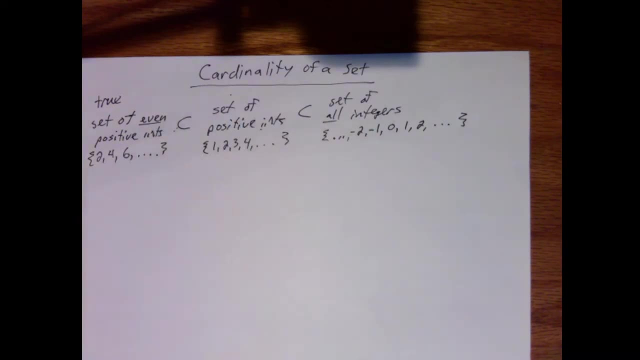 a subset of this. This is a subset of this, which means this is also a subset of this, And you're probably looking at it thinking, wow, this then must be smaller than this which is smaller than this, But in terms of cardinality that's not. 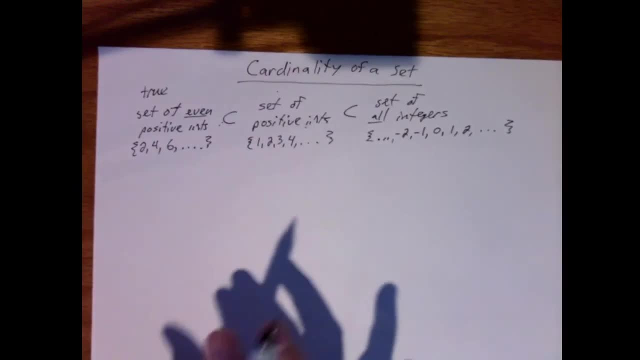 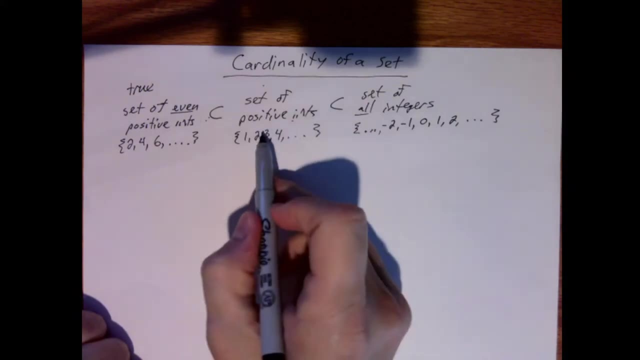 necessarily the case. So remember what we said: If we can find a bijection from the set of positive integers to some other set, then they have the same cardinality, And what that means is coming up with a way of mapping every one of these numbers to the numbers. 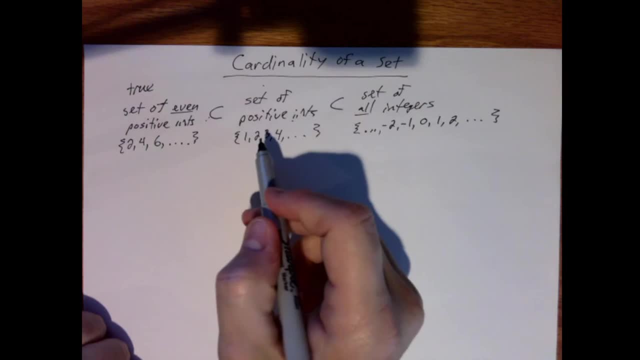 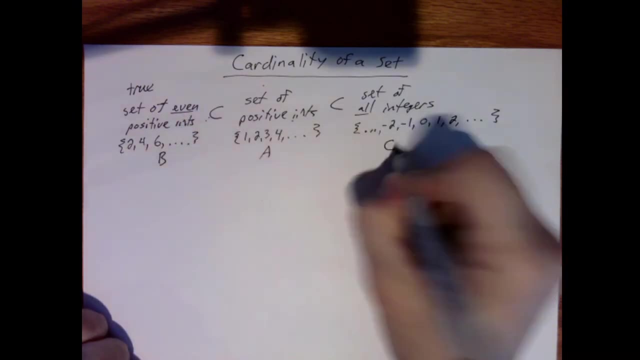 in the other set or the elements in the other set. I guess it wouldn't necessarily have to be numbers. All right, So let's say here we'll call this set A, set B and set C, just to make it easy to distinguish between what I'm talking about. So A will be the set of 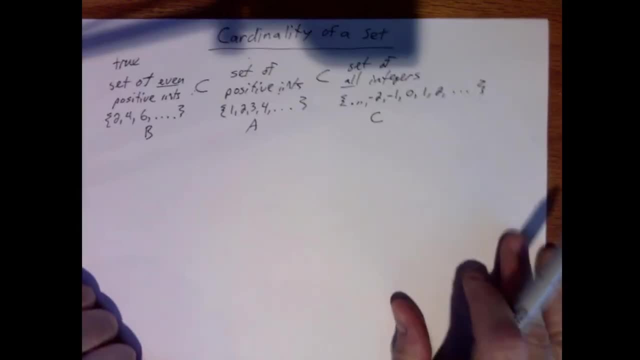 positive integers. B will be the set of even positive integers And C will be the set of all integers, And really this is let's just show you. So this is the set of even positive integers, And C will be the set of all integers, And really this is let's just show you. So this is the set of even positive integers, And really this is the set of all integers, And really this is the set of all integers And really this is the set of all integers. Let's just show you something quick, just to do this. This is z, because that's. 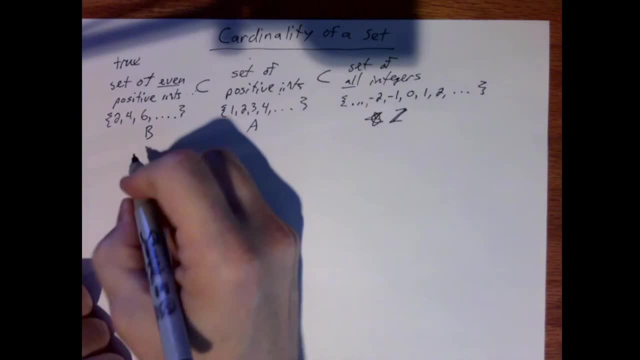 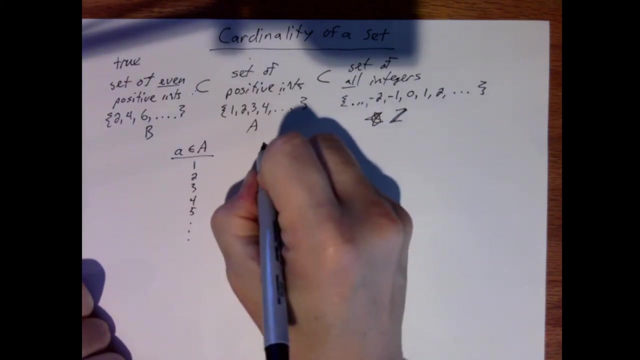 the standard way of talking about it. So if I were to have that, a was an element of set a right, so we'd have 1,, 2,, 3,, 4, 5,, dot, dot, dot. What if I were to write down 2a? 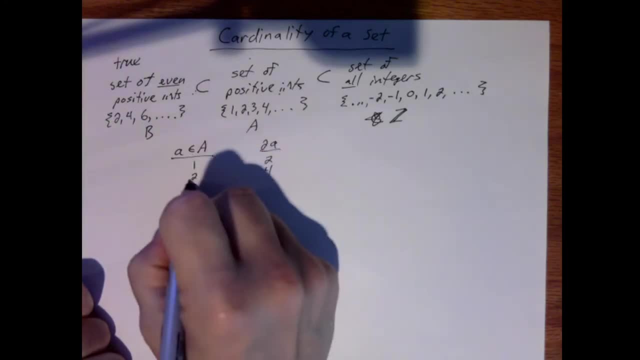 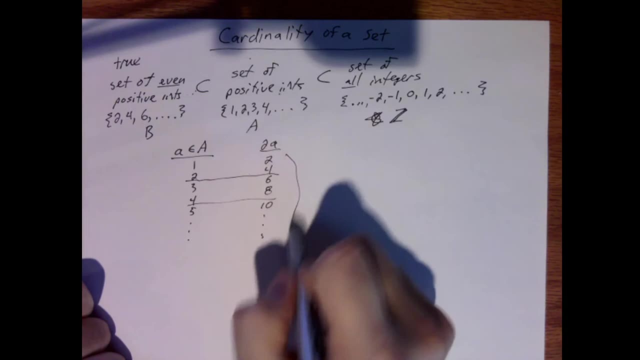 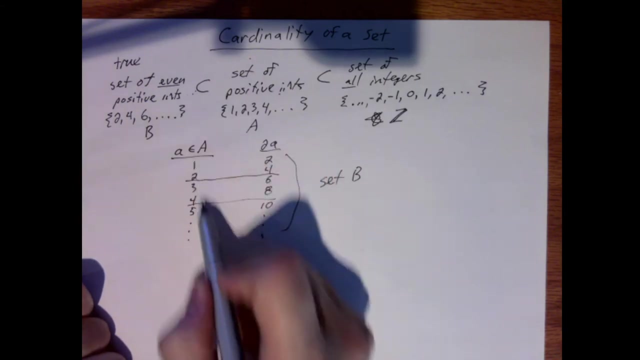 Well, 2a would be 2,, 4, and we'll put some lines here to keep them straight: 6,, 8,, 9,, 9,, 10, and 11.. 10, dot, dot, dot. well, this right here is set b. i just found a mapping. so that way, for every integer. 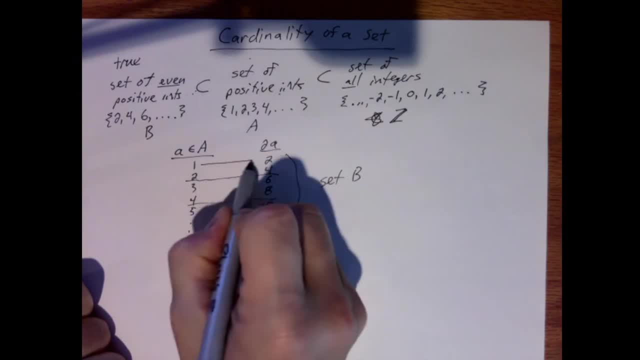 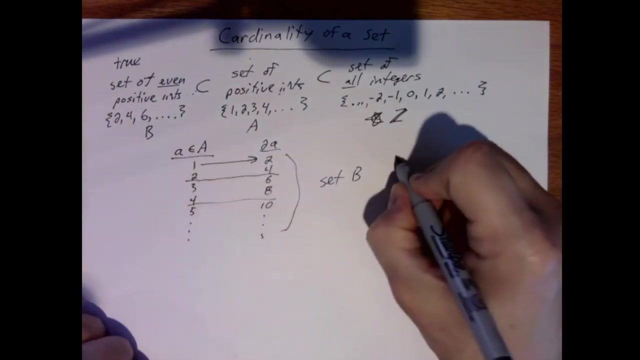 in the set of positive integers. i can show how to get to one of the elements of set b and i can go back the other way. we could take one half of these numbers and come back this way. so therefore i have the bijection and that means that the cardinality of a is equal to cardinality. 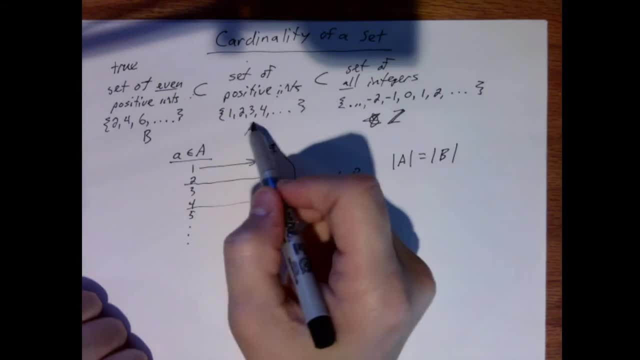 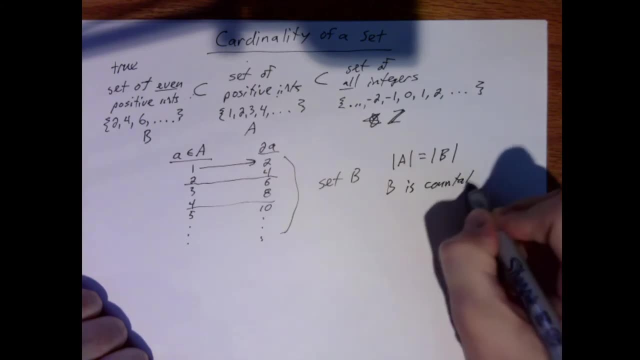 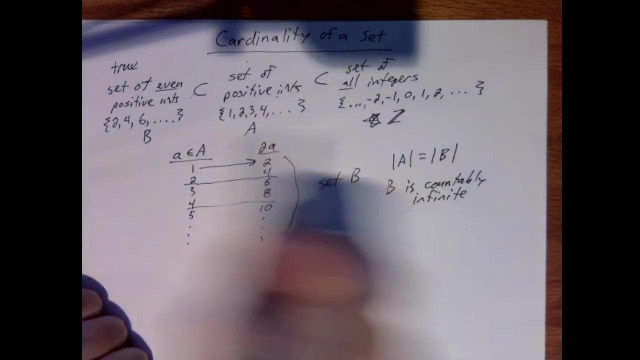 b and the set of positive integers happens to be countably infinite, so that means that b is countably infinite. all right, it's probably messing with your head. you're looking at this saying, yeah, but you skipped every one of these numbers, so how could this be the same as this? 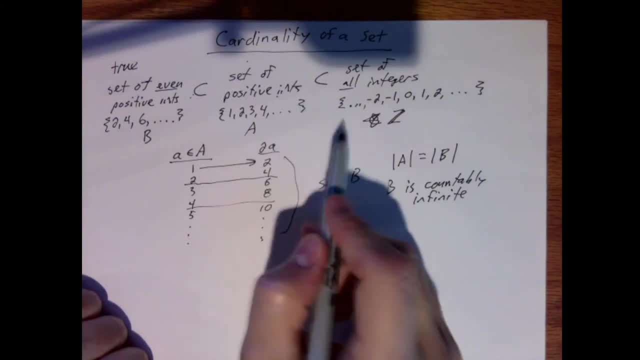 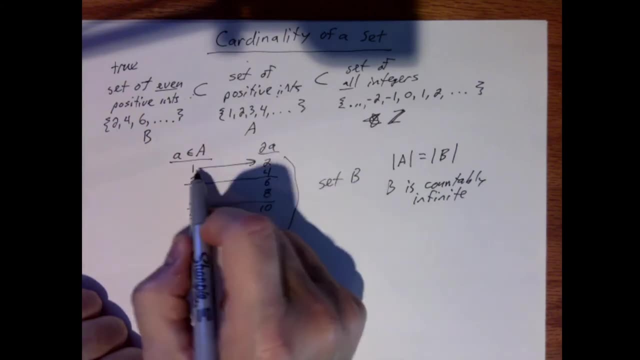 you. It goes back to the definition about the bijection. okay, If this is a set and this is a set, I can get to every one of these elements from a single value over here, And that's where the bijection comes in. 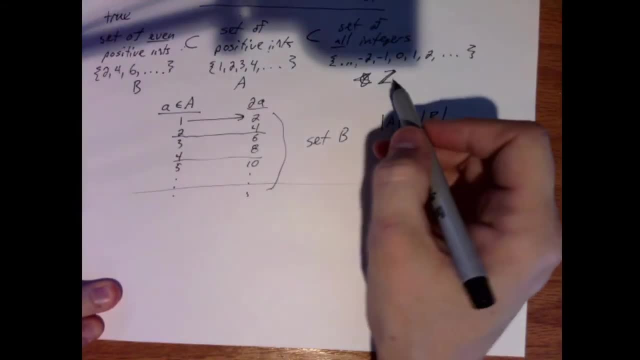 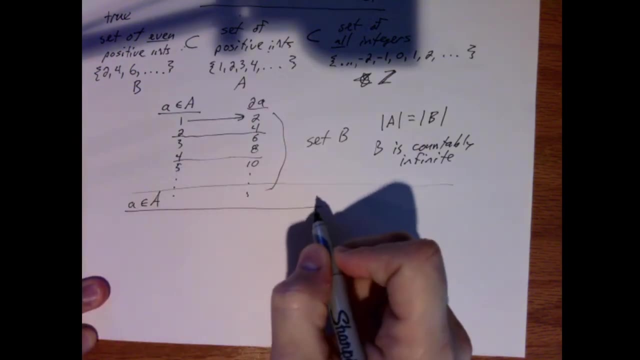 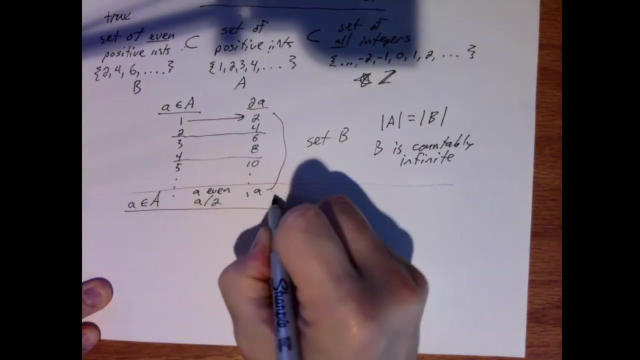 What about set Z? Okay, so once again, if I have a little, a is an element of set A And if a is even, I'm going to produce a divided by 2.. And if a is odd, I'm going to produce the negative of a minus 1 divided by 2.. 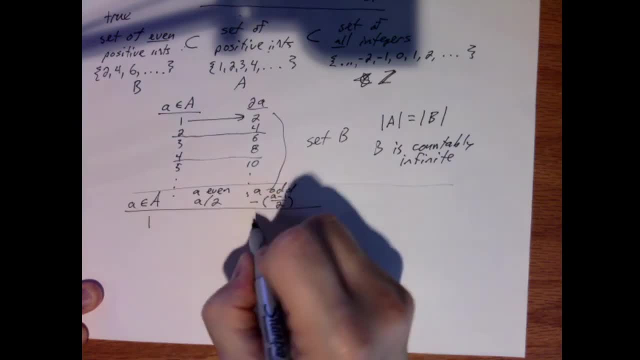 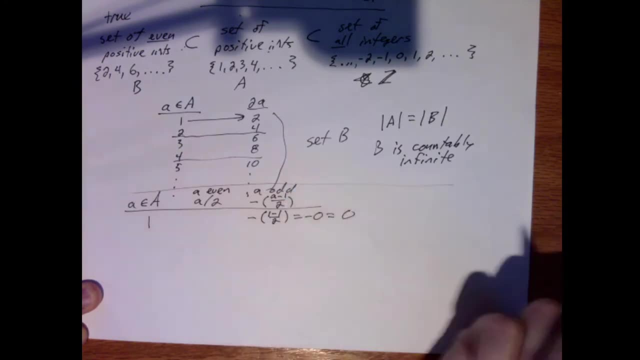 So when a is 1, that's odd. So I have minus 1, minus 1 over 2, which is minus 0, which is really just 0.. For 2, that's even. So I have: 2 divided by 2 is 1.. 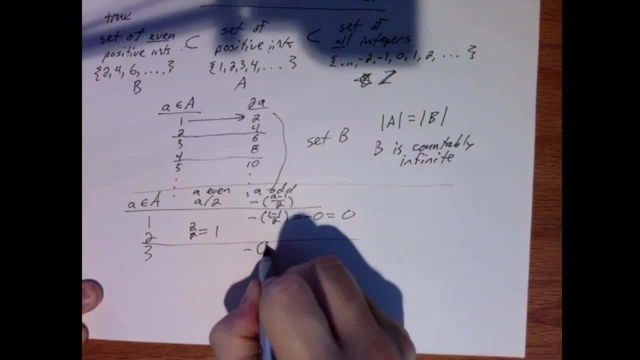 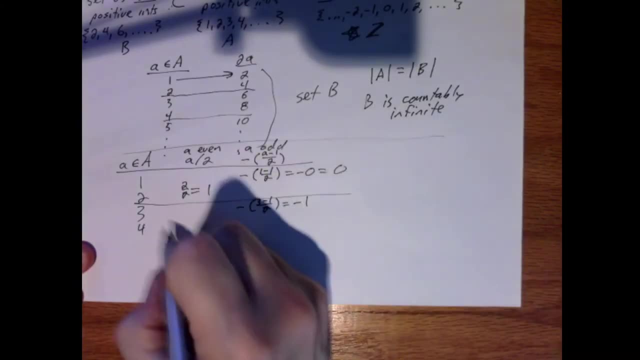 3, this would be now minus 3 minus 1, divided by 2, is equal to negative 1.. 4, that's 4 divided by 2, is 2.. 5 minus 5 minus 1 divided by 2.. 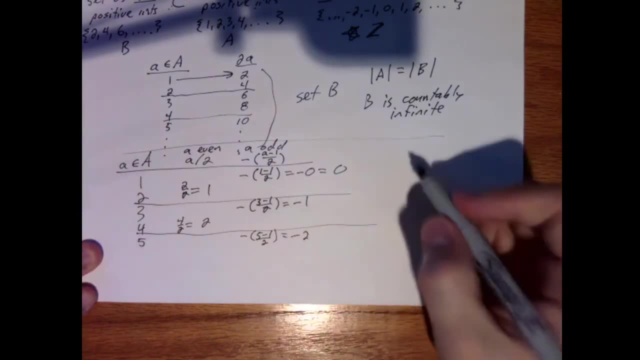 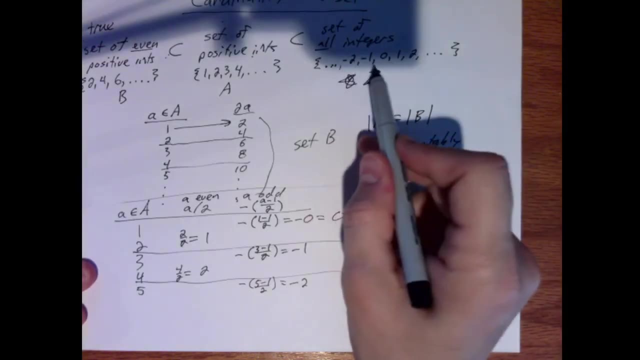 So that's minus 2.. So what am I producing here? Well, I don't have to write the integers in order to represent the set. I just need to be able to represent everything there. So what I'm producing here is this set. 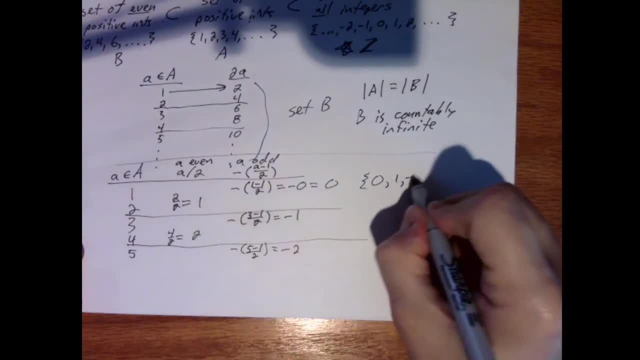 0, positive, 1, negative, 1, 2, negative, 2.. And then you can see how I'm just continuing. So this right here is the set of all integers, which means the set of all integers is counterintuitive. 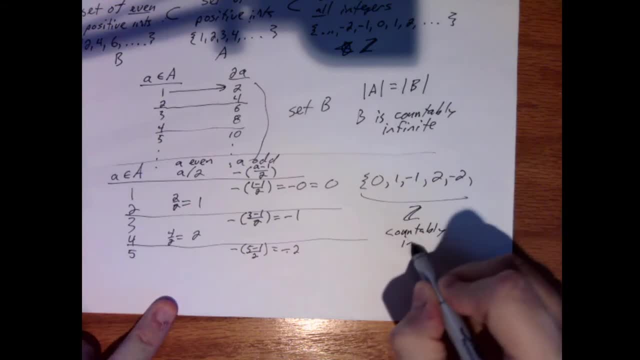 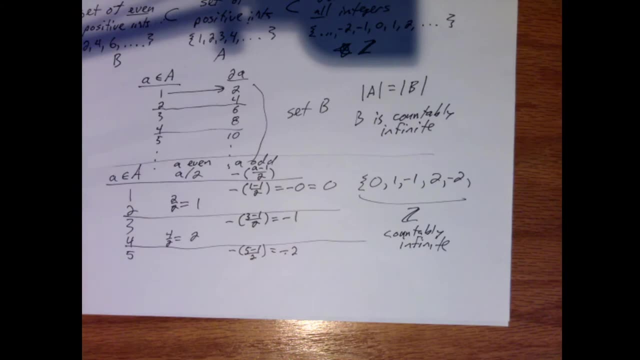 So that's because the set is terminally infinite. Let that sink in for a minute because it may be hurting your head. But, like I said, once again, it goes back to the definition of the bijection between the set of positive numbers and the set that we're looking at. 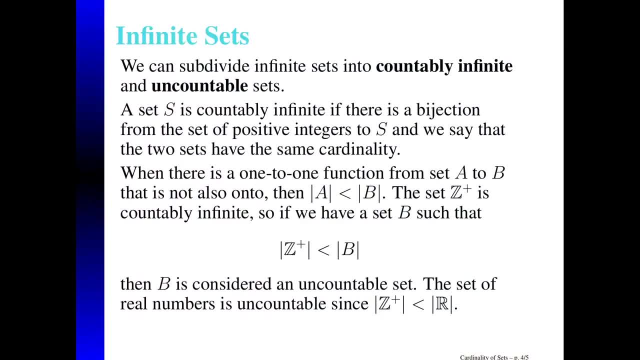 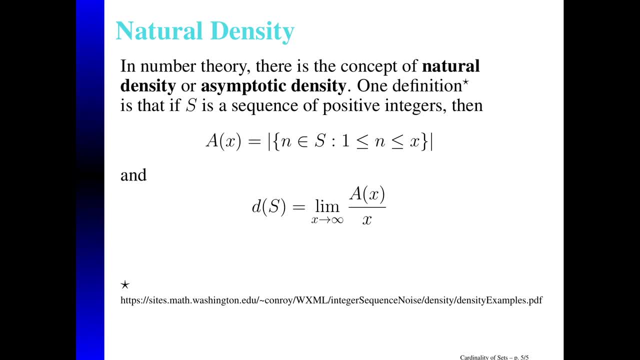 Okay, Okay. So now you still may be thinking. my gut still tells me me that, for example, the set of even positive integers has to have fewer elements than the set of all positive integers. right, Since I didn't write down the odd ones, Well, there is a concept. 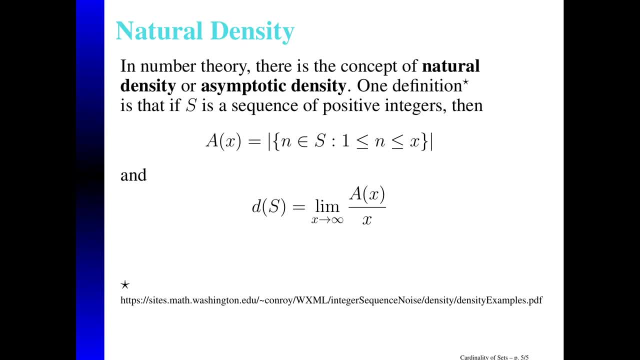 in number theory that's closer to what your intuition would be, And that idea is called the natural density or the asymptotic density, right, So you can find different definitions online and sometimes also talk about the lower asymptotic density or the upper asymptotic density. 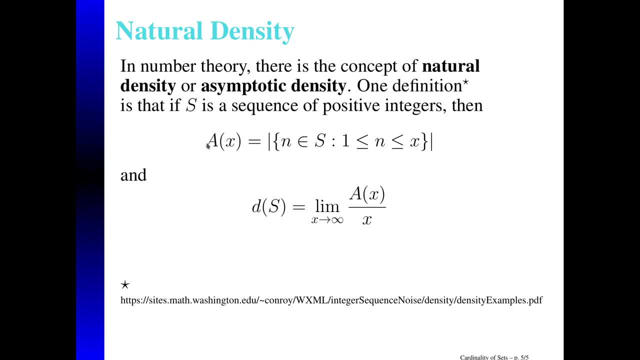 But this definition which I got from here, is talking about- see the vertical bars here- a of x will be the cardinality of the set, where if s is a sequence of positive integers and we choose those elements in the range of 1 to x, okay and take its size, the cardinality. 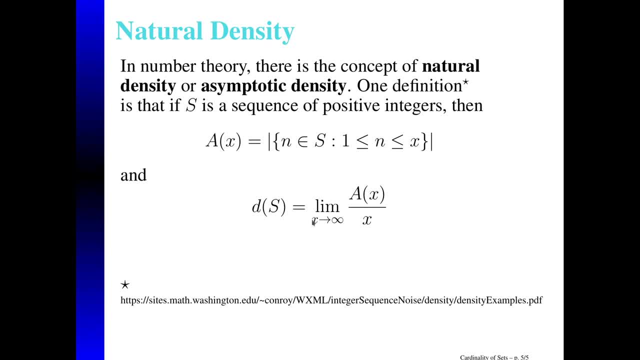 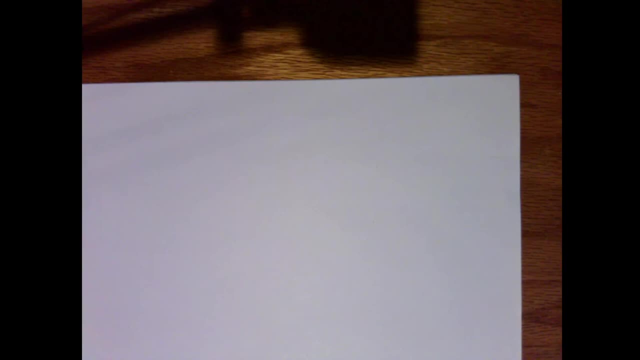 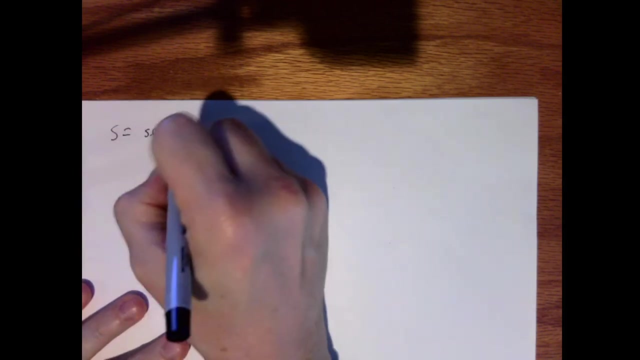 then if I were to take the ratio of that to x, as x approaches infinity, this will give me an idea of the density. So what does that mean? Well, let's say, for example, that we say s is the set of even positive. 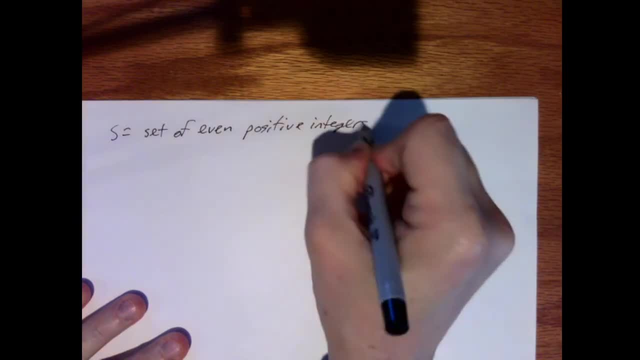 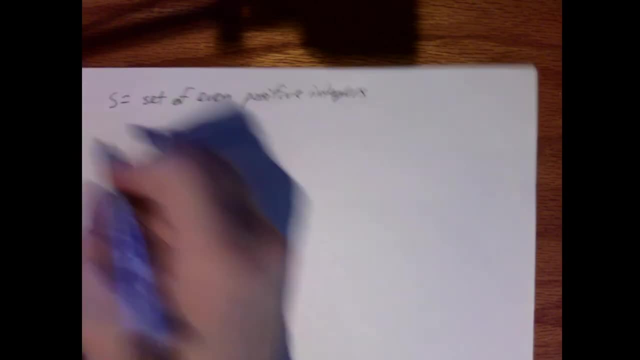 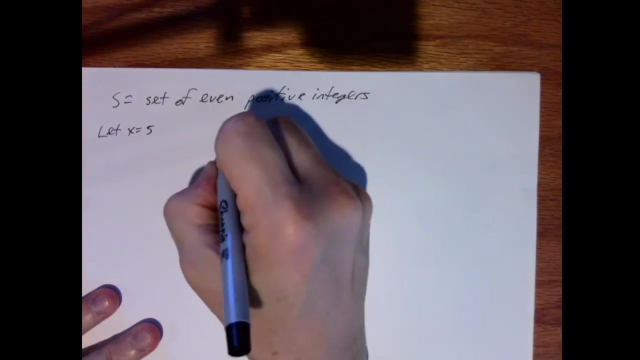 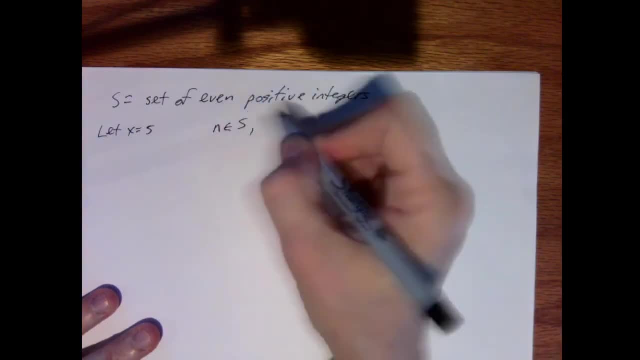 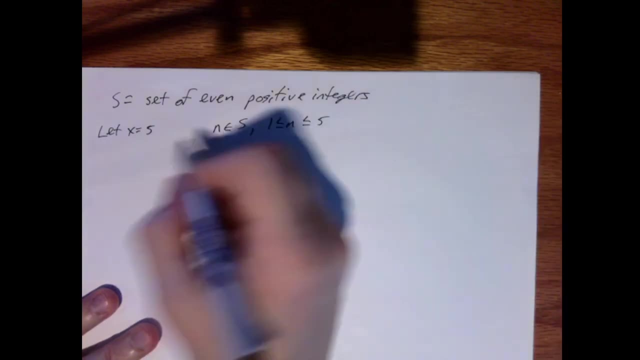 if n is an element of s and we're looking at the range of n is less than or equal is in the range between 1 to 5, then what we're producing here is this subset of s that would be 2 & 4. right, because the set of even integers will be. 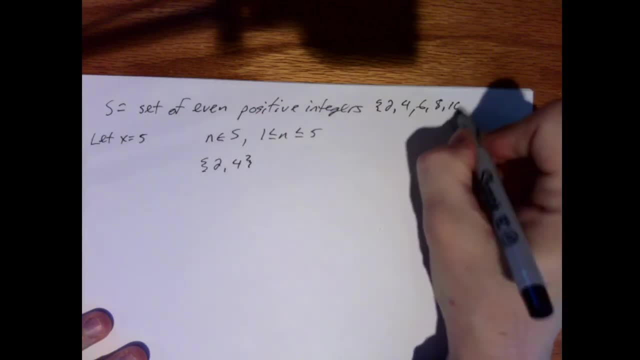 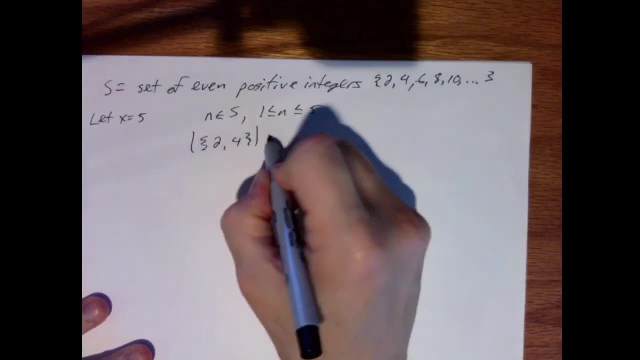 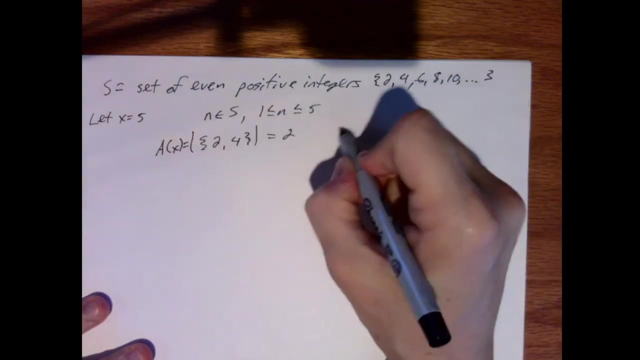 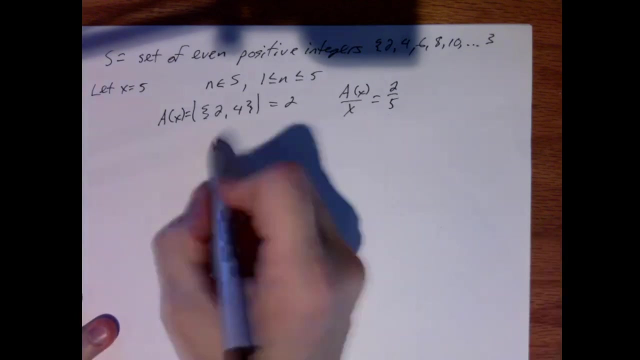 two, four, six, eight, ten, dot, dot, dot forever. so what happens if I take the cardinality of this? cardinality of that is 2, if I take the ratio of this. so what we just produced is ax. ax to x would be 2 fifths. okay, so now if we use the